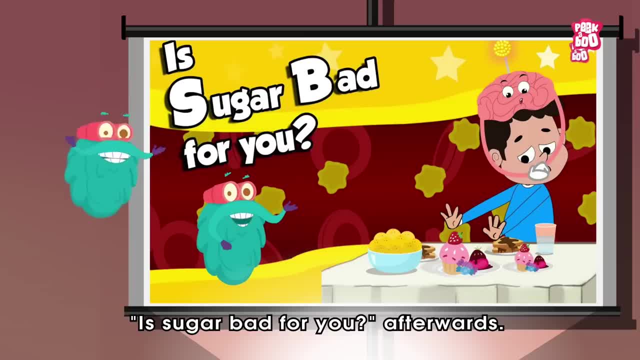 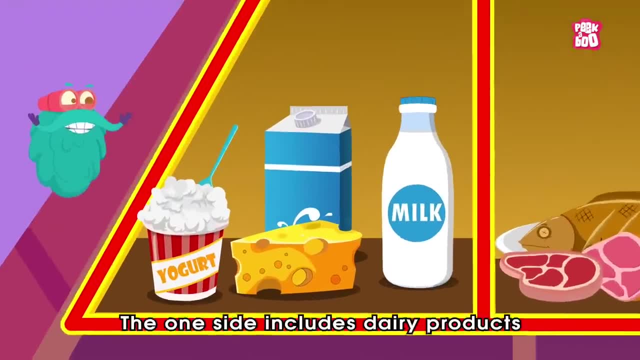 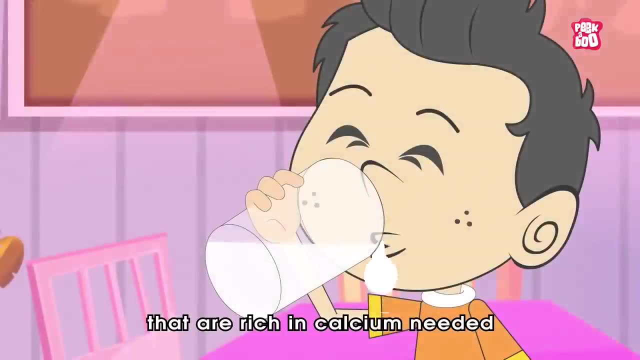 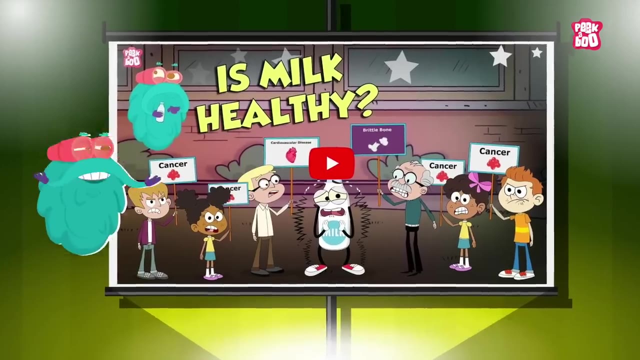 Is Sugar Bad For You afterwards? The second section of the pyramid is further divided into two groups. The one side includes dairy products like milk, yogurt and cheese That are rich in calcium, needed for strong bones and teeth. But before deciding to consume milk. 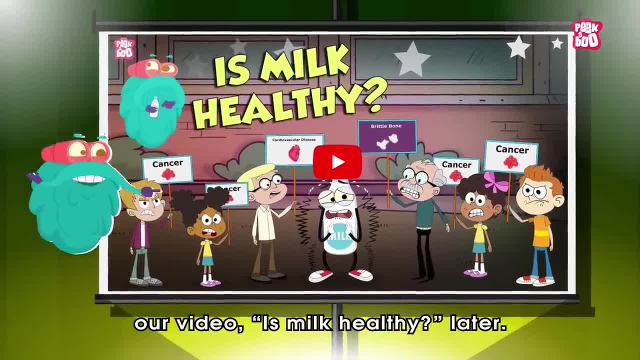 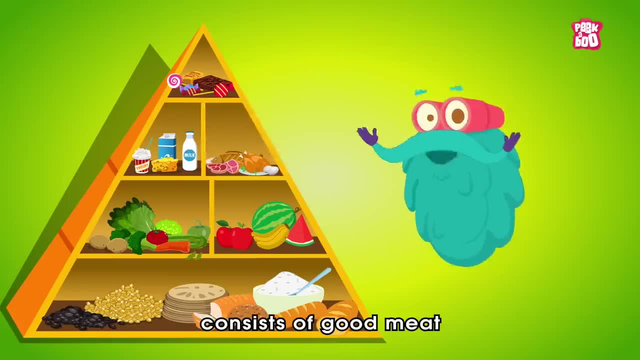 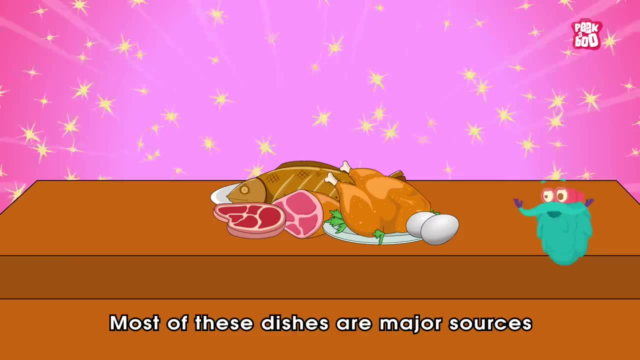 we would request you to please check out our video. Is Milk Healthy later? And the other side of section two consists of good meat like chicken, turkey fish and eggs. Most of these dishes are major sources of proteins, zinc and protein. 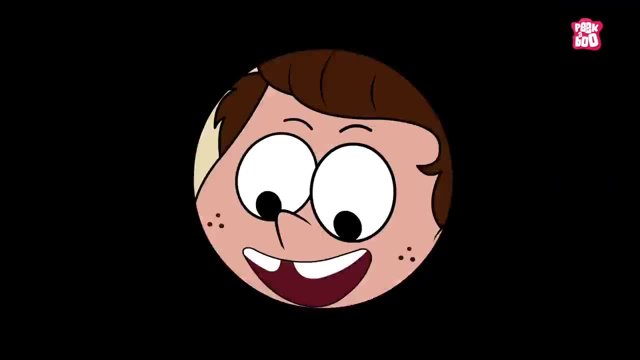 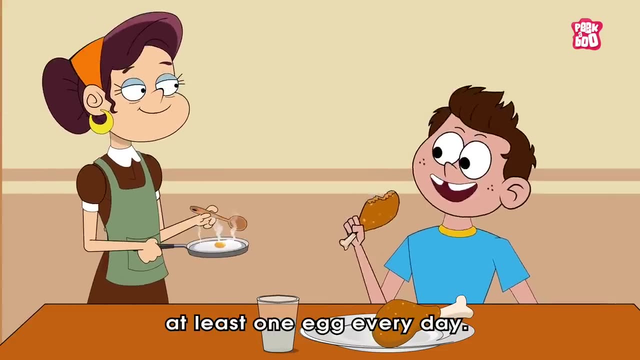 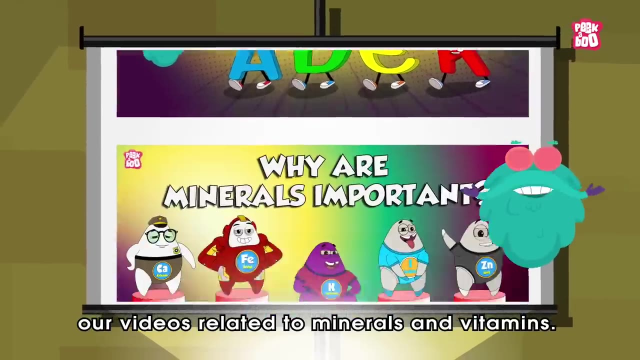 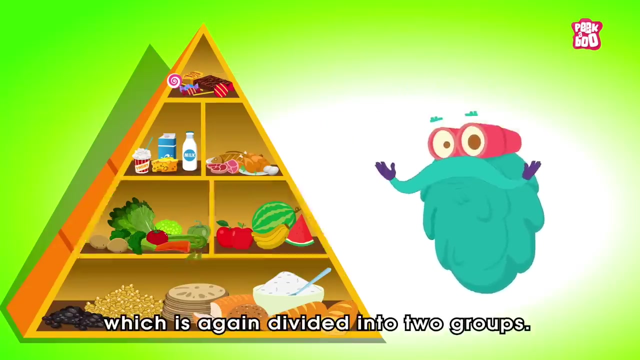 Needed for our growth and development. Hence it is recommended to have at least one egg every day. Again, to know more, please check out our videos related to minerals and vitamins. Now let's move to the third section, which is again divided into two groups. 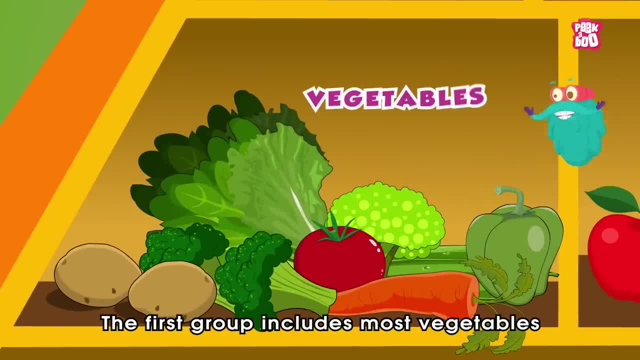 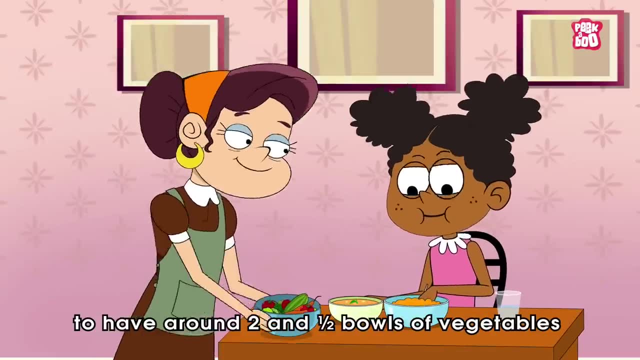 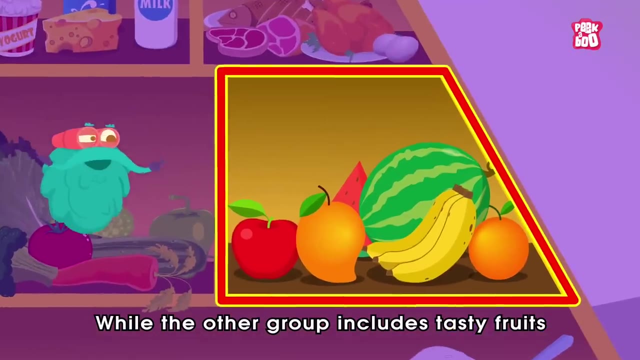 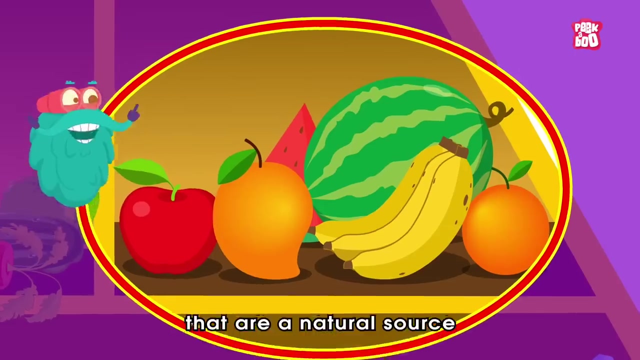 The first group includes most vegetables that are a healthy source of nutrition, due to which it is recommended to have around two and a half bowls of vegetables every day, While the other group includes tasty fruits like apple, orange, banana, mango, etc. that are a natural source of sugar, fiber and vitamins. 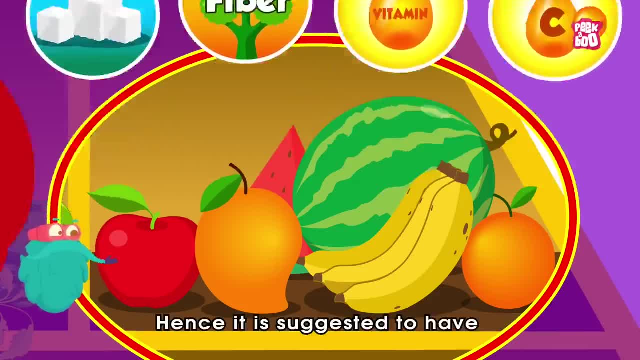 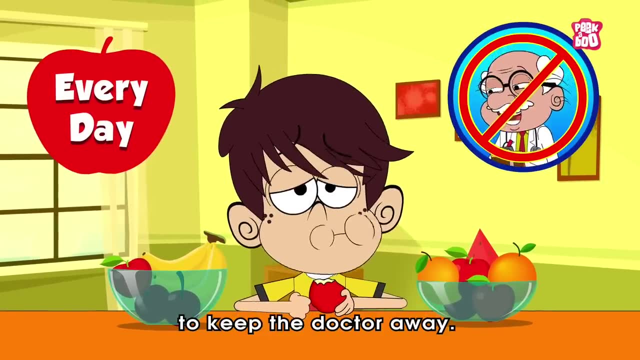 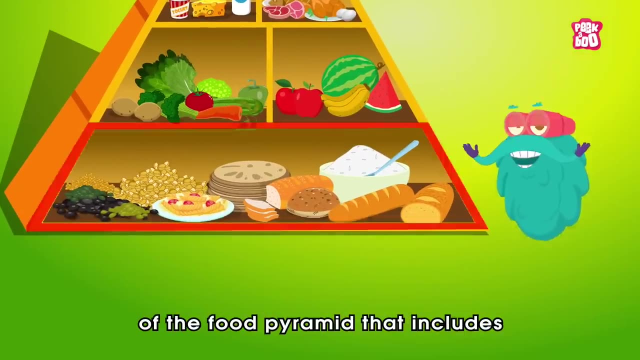 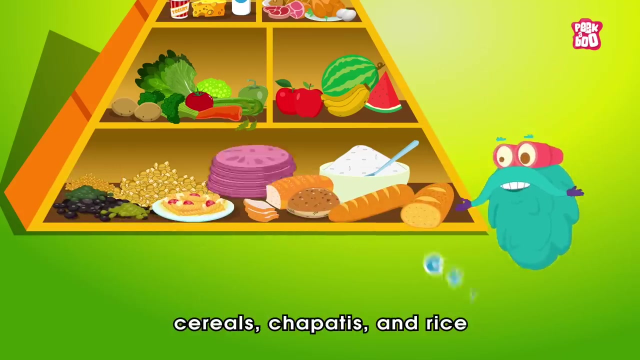 especially vitamin C. Hence it is suggested to have two bowls of fruits every day to keep the doctor away. Finally comes the fourth, the base and the biggest section of the food pyramid. that includes all grains: lentils, bread, pasta, cereals, chapatis and rice. 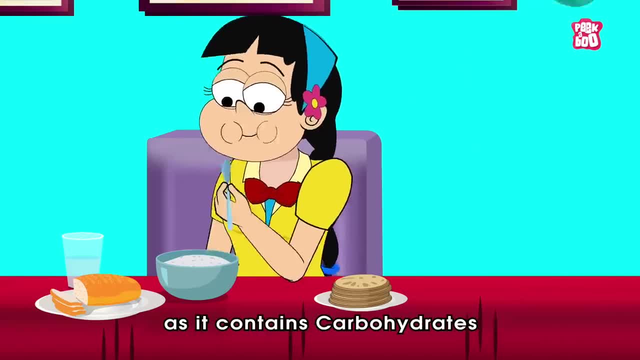 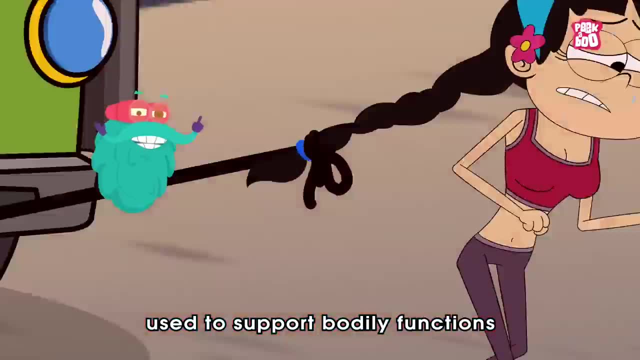 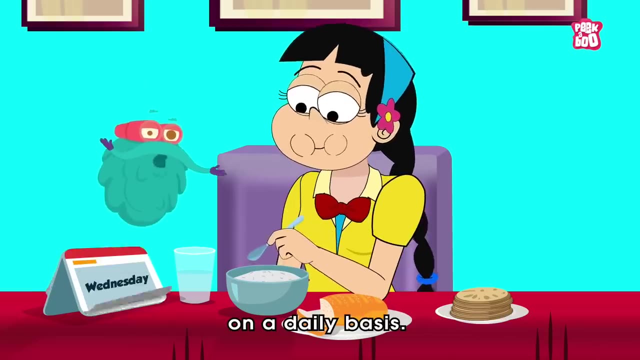 This is a very important food group, as it contains carbohydrates that provide the body with glucose, which is converted to energy used to support bodily functions and physical activity. Hence, it is recommended to eat them on a daily basis. So here we go, my friends.